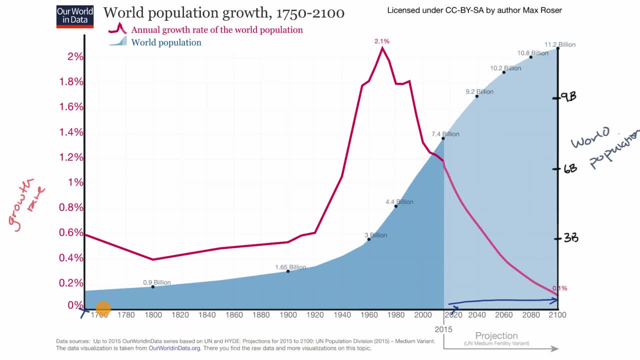 One. you might just wonder: well, what was the world population around 1750?? And if you look at this- and these are obviously estimates because you did not have a global census back in 1750, it was around seven or 800 million people. 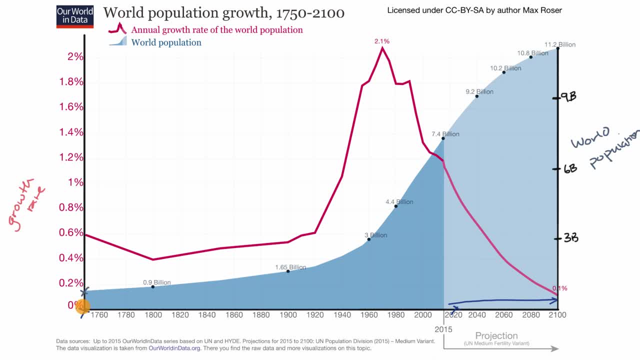 Now what's interesting is that's not a lot larger than the number of people that we had at, say, the time of Jesus, which is also the time of the Roman Empire, and Han China, where it's estimated that at around that time period, 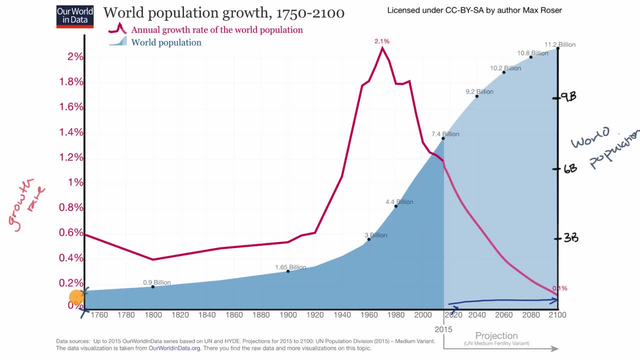 around 2000 years ago the world population was around 300 million people. But then we see something interesting happen: Over the next several centuries- from 1750, it seems to start growing pretty dramatically, And we could see why that is. 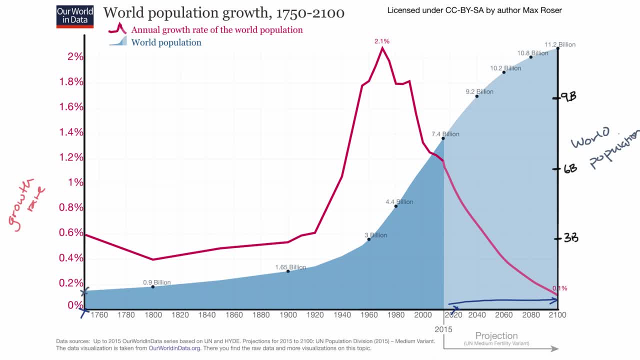 We can see the growth rate of population For a while if we look at this red curve. the growth rate of world population was around 0.6%, but it looks like in the early 20th century right around here. the rate of growth of world population. 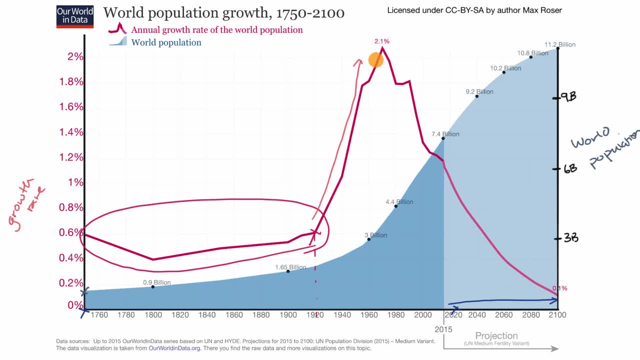 starts to really increase where, at least based on this, it looks like around the 1970s world population, the growth rate peaked out at 2.1%. Now the question might be: why was this happening? Why did the rate of growth increase so much? 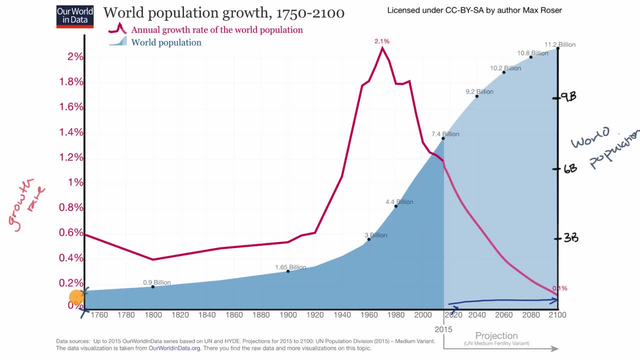 around 2000 years ago the world population was around 300 million people. But then we see something interesting happen: Over the next several centuries- from 1750, it seems to start growing pretty dramatically, And we could see why that is. 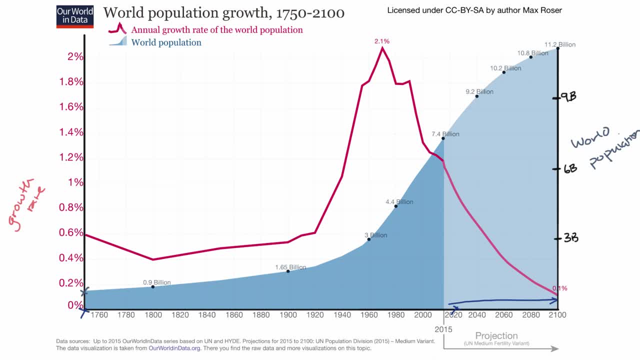 We can see the growth rate of population For a while if we look at this red curve. the growth rate of world population was around 0.6%, but it looks like in the early 20th century right around here. the rate of growth of world population. 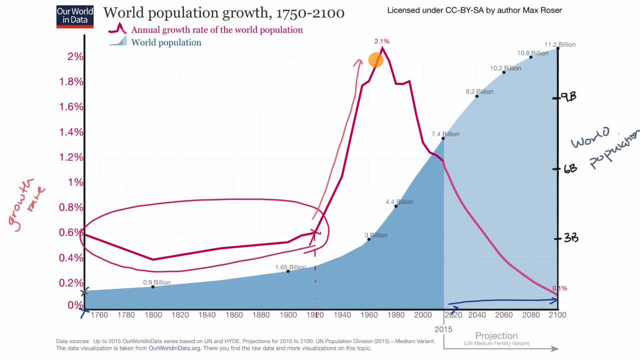 starts to really increase where, at least based on this, it looks like around the 1970s world population, the growth rate peaked out at 2.1%. Now the question might be: why was this happening? Why did the rate of growth increase so much? 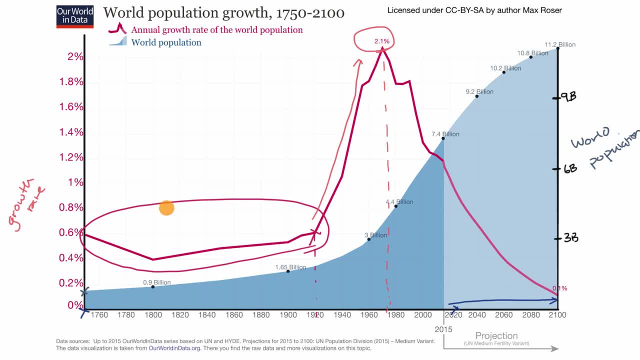 Well, the main argument is: as we became a more industrial society, healthcare would have improved, So child mortality would have gone down. People would have died of fewer diseases. At the same time, we would have gotten more efficient with agriculture. we would have had modern farming methods. 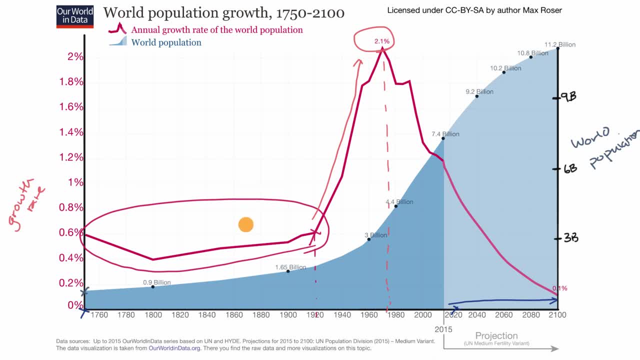 So more people. so food would get cheaper, it would be more abundant, more people would have access to nutrition, And all of those would drive the growth rate up. Now an interesting question that folks have been thinking about for many hundreds of years. 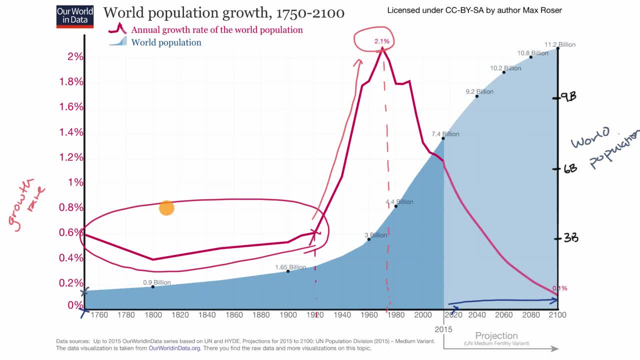 Well, the main argument is: as we became a more industrial society, healthcare would have improved, So child mortality would have gone down. People would have died of fewer diseases. At the same time, we would have gotten more efficient with agriculture. We would have had modern farming methods. 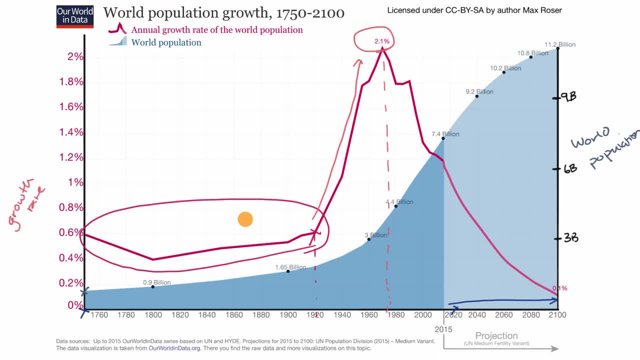 So more people. so food would get cheaper, It would be more abundant, More people would have access to nutrition, And all of those would drive the growth rate up. Now an interesting question that folks have been thinking about for many hundreds of years. 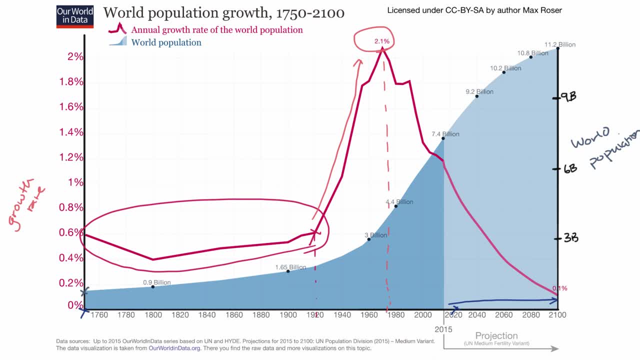 is there a limit to how much human population the Earth can sustain, And so they've introduced this idea known as carrying capacity. Why do we use the letter K for capacity When capacity starts with a C? because a version of that word in German starts with a K. 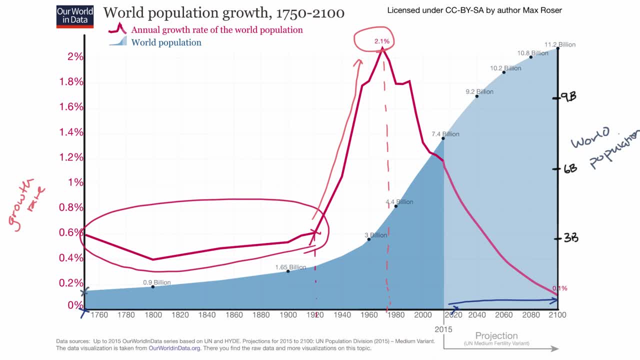 is there a limit to how much human population the Earth can sustain, And so they've introduced this idea known as carrying capacity. Why do we use the letter K for capacity? When capacity starts with a, K, it's carrying capacity. When capacity starts with a, C. 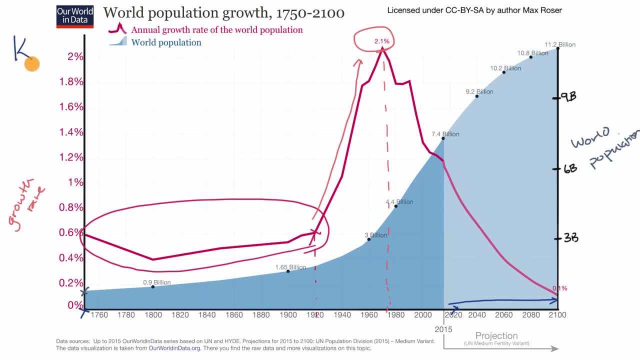 because a version of that word in German starts with a K, And there's always been this notion that for a given species there's gotta be some maximum capacity that an ecosystem can sustain. And there's folks like Thomas Malthus who's theorized that there must be some limit. 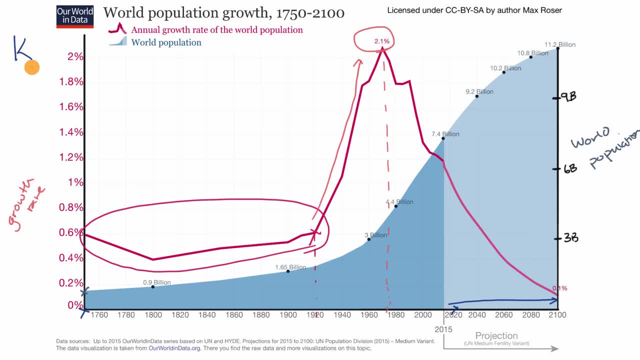 to how many people there could be on the planet just based on how much land there is, how much nutrition or how much resources there are. But the carrying capacity for humanity is really an open question Because our technology is constantly on the move. 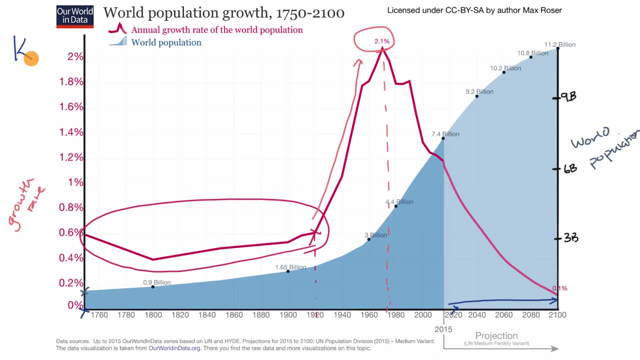 And there's always been this notion that for a given species there's gotta be some maximum capacity that an ecosystem can sustain. And there's folks like Thomas Malthus who's theorized that there must be some limit to how many people there could be on the planet. 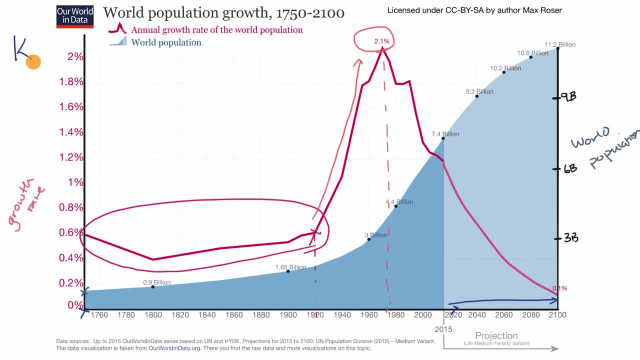 just based on how much land there is, how much nutrition or how much resources there are. But the carrying capacity for humanity is really an open question because our technology is constantly on the move. We constantly are getting better at using our resources more efficiently. 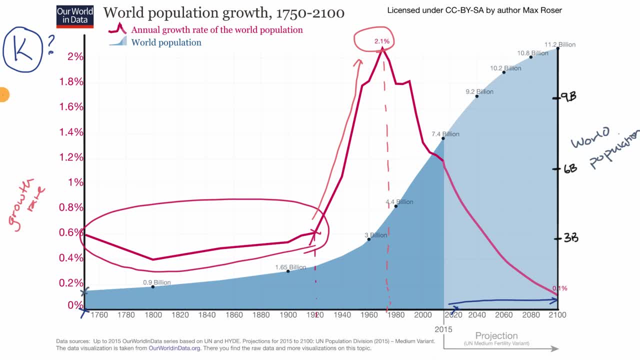 going into new ecosystems. Now it's a huge debate: how sustainable is that? And as we become more efficient, are we also trashing certain parts of our ecosystem? But the carrying capacity of humans? we really don't know how many people. 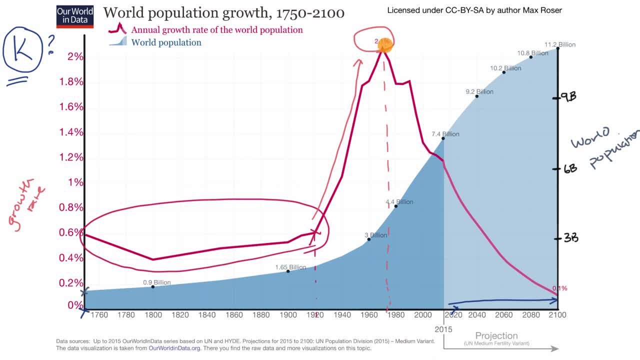 the planet Earth could sustain, But we could see that the rate of population growth starts to decline after 1970. And the main argument for this- and we see this and we cover this in other videos- when we study countries that are still developing and countries that would be considered industrial- 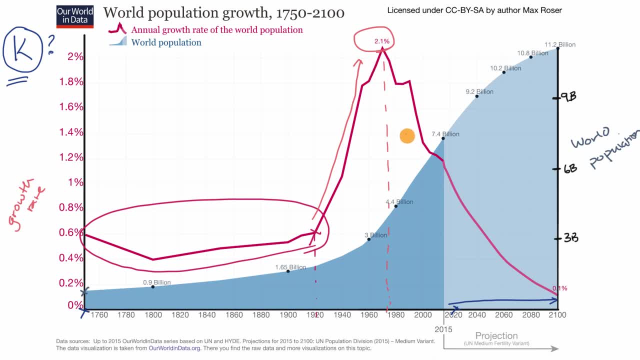 or even post-industrial, is that as countries develop and become wealthier, you might have more women entering into the workforce. you might have more family planning. women have more control over their destiny, get education longer and people just have fewer children. 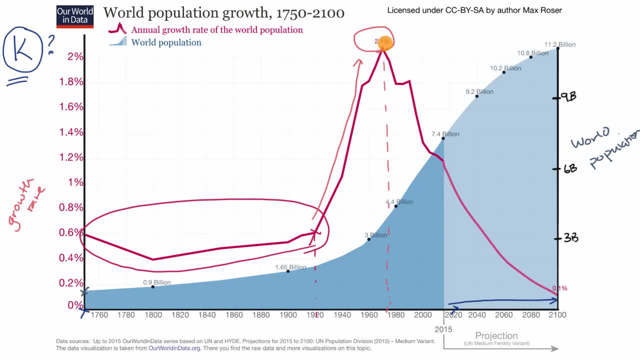 And so, as people have fewer children- you could see that the world, that especially we see this in industrial and post-industrial countries- the growth rate starts to come down, And so the aggregate growth rate is coming down, arguably because more and more countries are becoming wealthier. 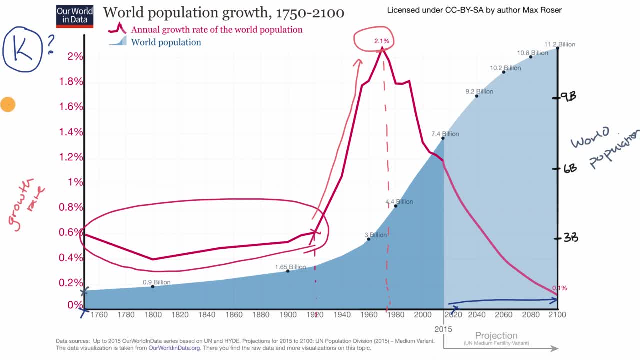 We constantly are getting better at using our resources more efficiently, going into new ecosystems. Now it's a huge debate: how sustainable is that? And as we become more efficient, are we also trashing certain parts of our ecosystem? But the carrying capacity of humans? 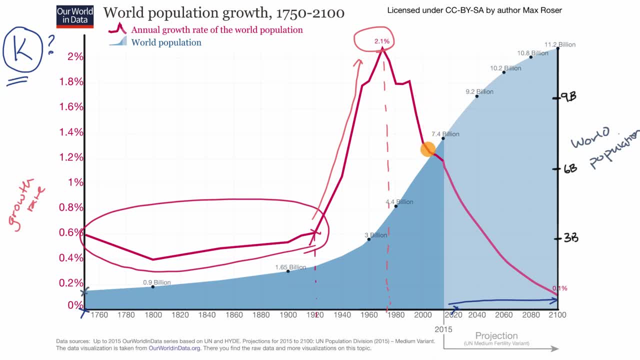 we really don't know how many people the planet Earth could sustain, But we could see that the rate of population growth starts to decline after 1970. And the main argument for this, the main argument for this- and we see this and we cover this in other videos- 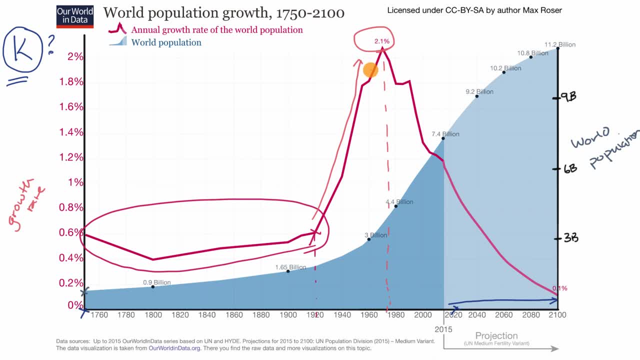 when we study countries that are still developing and countries that would be considered industrial or even post-industrial, is that, as countries develop and become wealthier, you might have more women entering into the workforce. you might have more family planning. women have more control over their destiny. 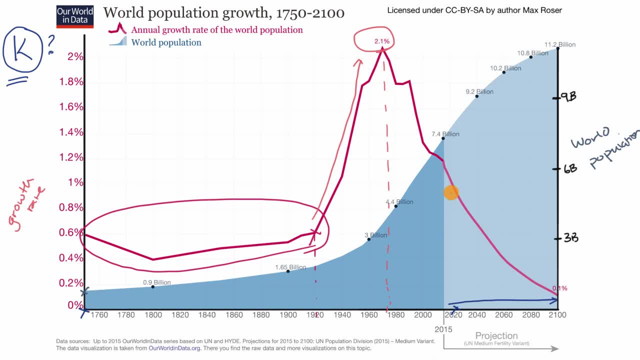 get education longer and people just have fewer children. And so as people have fewer children- you could see that the world, that especially we see this in industrial and post-industrial countries- the growth rate starts to come down, And so the aggregate growth rate is coming down arguably. 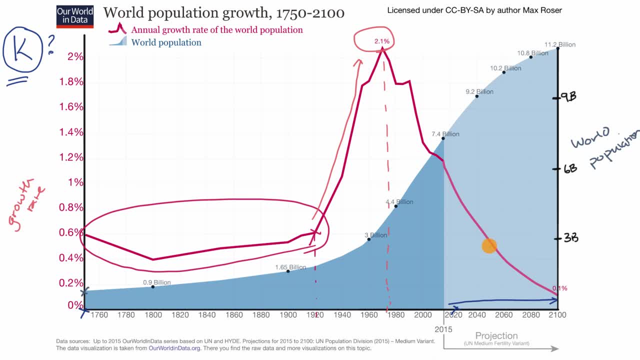 because more and more countries are becoming wealthier, have better healthcare, better rights for women, And we even see today that, when you look at countries that are developing, their growth rate is around 1.2%, while more economically developed nations are at around 0.2%. 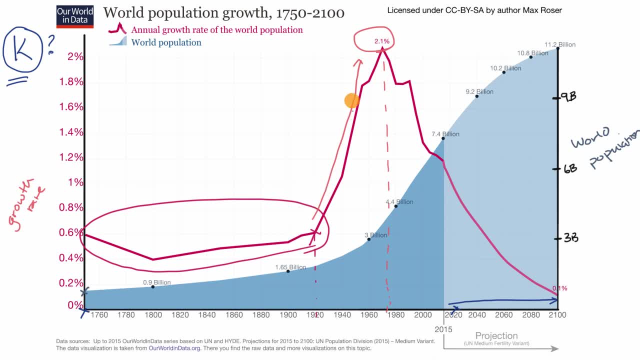 So there's definitely that correlation between the two, And, of course, this growth rate that you see in red is going to affect the absolute population, And so it's no coincidence that at the same time that the growth rate started to go up like that, 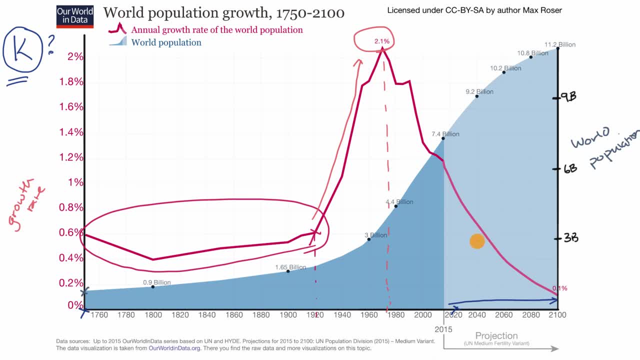 have better healthcare, better rights for women, And we even see today that, when you look at countries that are developing, their growth rate is around 1.2%, while more economically developed nations are at around 0.2%. So there's definitely that correlation between the two. 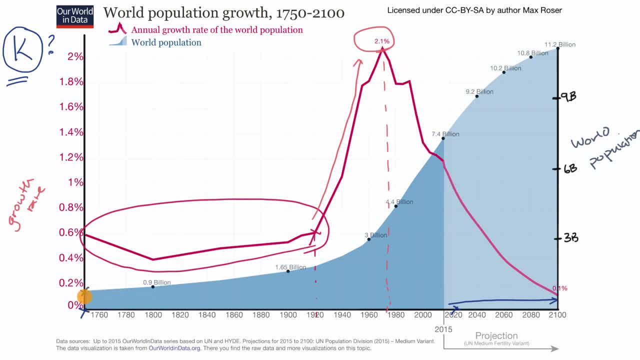 And, of course, this growth rate that you see in red is going to affect the absolute population, And so it's no coincidence that at the same time that the growth rate started to go up like that, we see that the population in absolute terms. 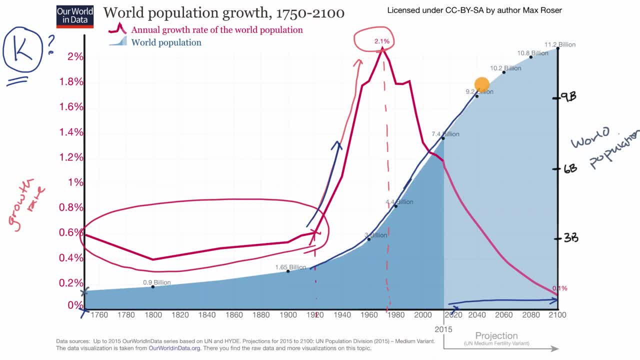 we see that the population in absolute terms starts to accelerate And just over, let's say, the last 100 years, we've gone from 1.65 billion, or I guess, if we go back 100 years, to 1920,. 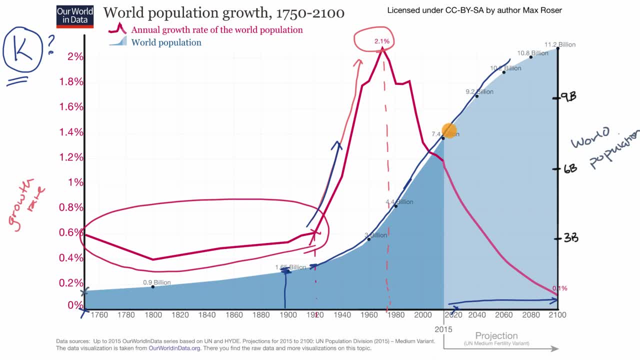 it looks like we're approaching 2 billion folks and now we're sitting at roughly 7.5 billion folks, So the world population roughly doubled over the, let's say, 2,000 years prior to this chart, But then, over this chart, over just the last 270 years.